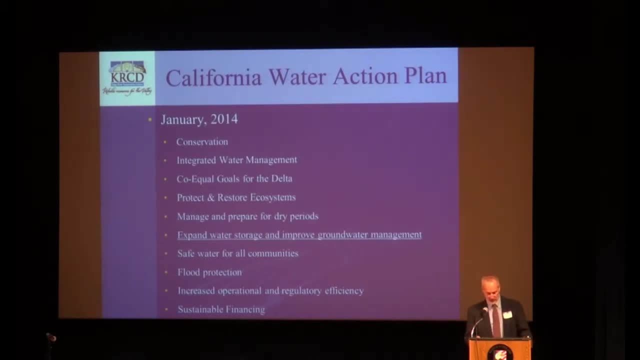 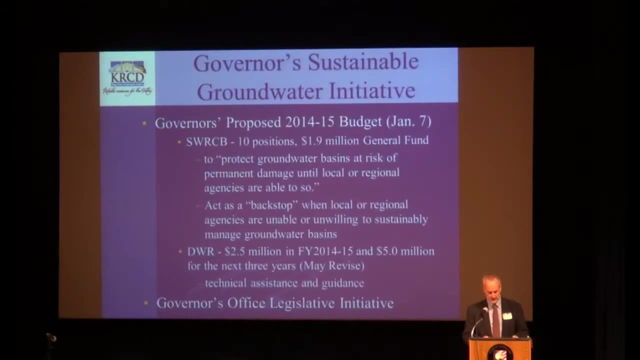 Or on this frame, is to expand water storage and improve groundwater management. It caused a lot of people to try to figure out what that means. The governor then initiated a sustainable groundwater initiative, which was a white paper that was supported by a couple of budgetary proposals and actions. 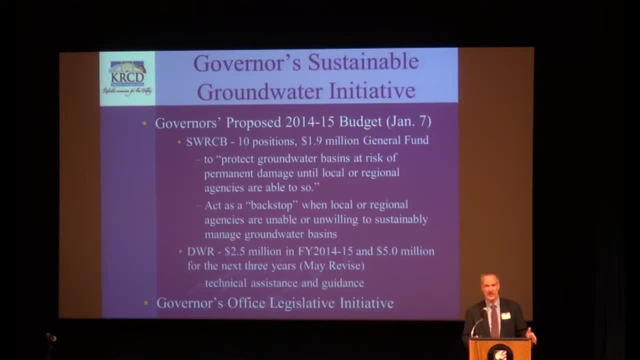 That included increased funding for the State Water Resources Control Board to get more involved in management of groundwater And then additional funding for the Department of Water Resources to continue their role in collecting technical information. That all evolved into a legislative initiative that was offered out of the governor's office late last year, early this year. 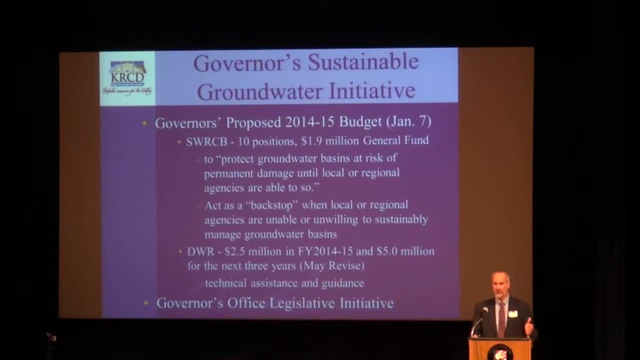 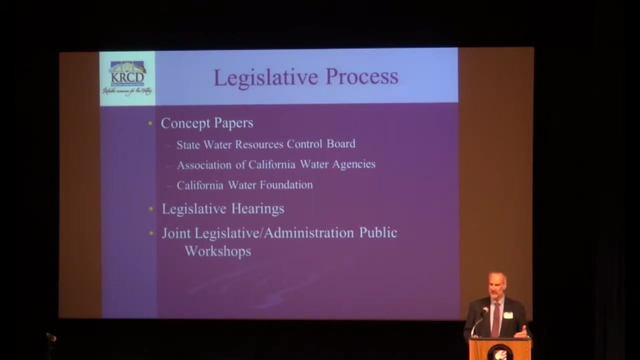 They set out some legislative concepts that were informed by both their California Water Action Plan and various agency input into some basic legislative objectives. The legislative process that ensued and really got moving in April- May, I guess- of this year, really started last fall with the development of some concept papers. 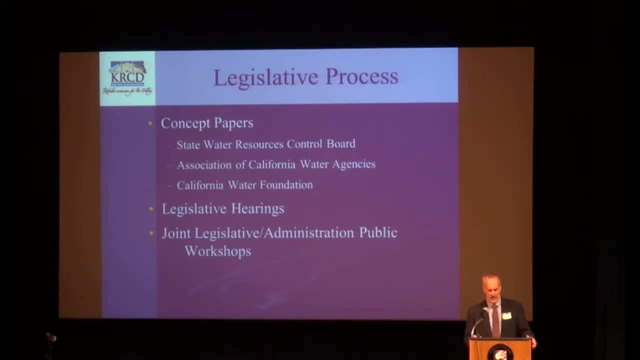 First there was a State Water Resources Control Board concept paper that explored an enhanced role that the State Water Resources Control Board could take in pushing groundwater management to some objective of I'll use the term sustainability And I'll define that a little bit better later. 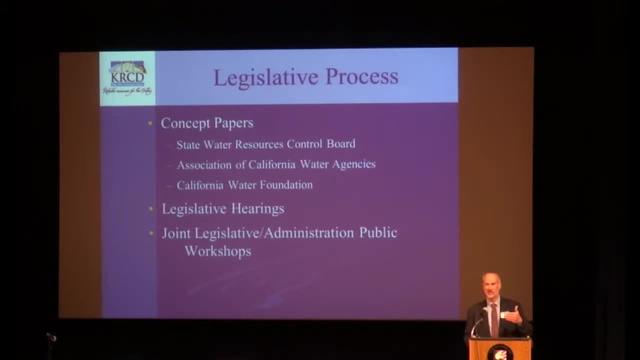 But simultaneously with that, in November of last year, the Board of Directors of the California Water Agencies, ACWA, initiated a groundwater task force that ultimately put together a policy paper, And concurrent with that was the efforts by the California Water Foundation to develop a policy paper. 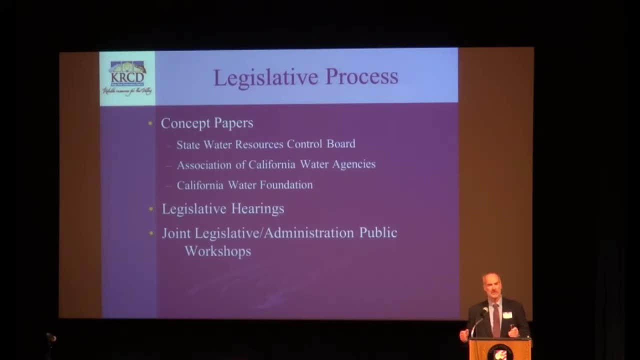 Those last two policy papers had a people referred to as a remarkable level of convergence. There was some agreement and some basic concepts, But within those, those then led into an effort to convert those policy papers to legislation, There were a number of legislative hearings conducted, albeit pretty thin, frankly, looking back. 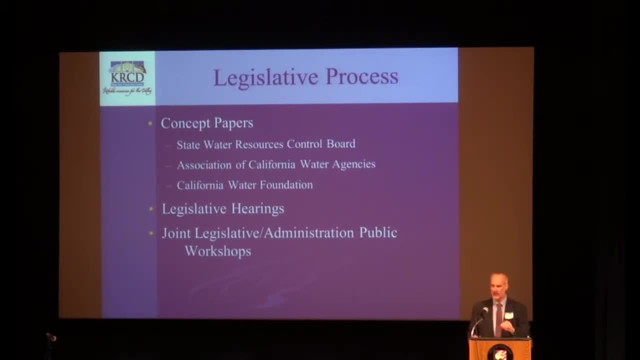 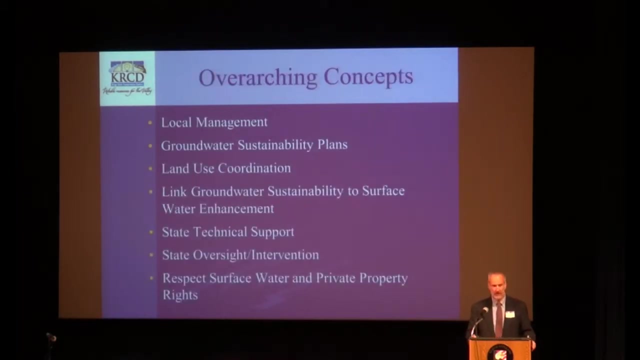 The process was moving very, very quickly in some venues, And so the administration and legislators brought to the public some specific policy questions, asked input of the public on those specific issues, and then took that input back into further drafting Some overarching concepts that came out of both the Water Foundation and the ACWA paper. 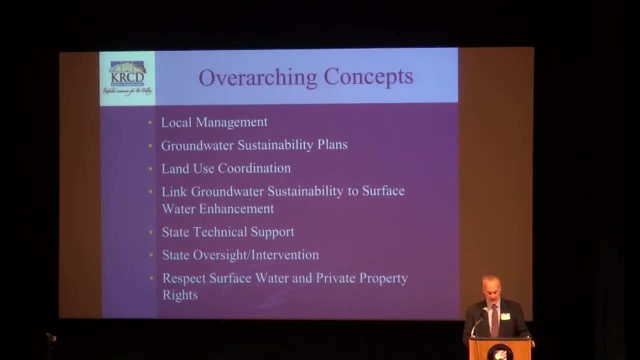 and, frankly, some of these are very much directed by efforts within the Kings River service area. I became deeply involved in this, mainly because our Board of Directors at KRCD, in coordination with the Kings River Water Association, felt that the risk was too high to let that happen. 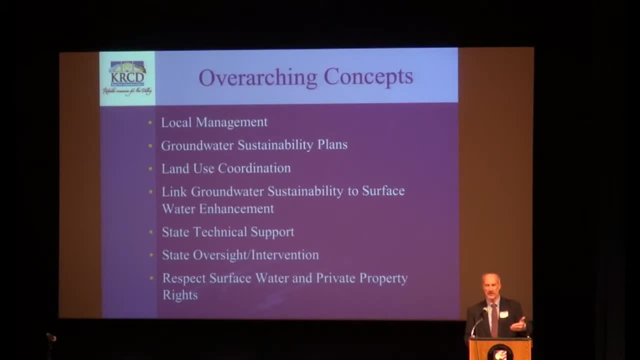 They felt that the risk was too high to let the legislature do this on their own, And so I'm very supportive of some basic objectives that were incorporated into these policy papers and ultimately, in part, in the legislation- and I emphasize, in part. We didn't get everything we asked for. 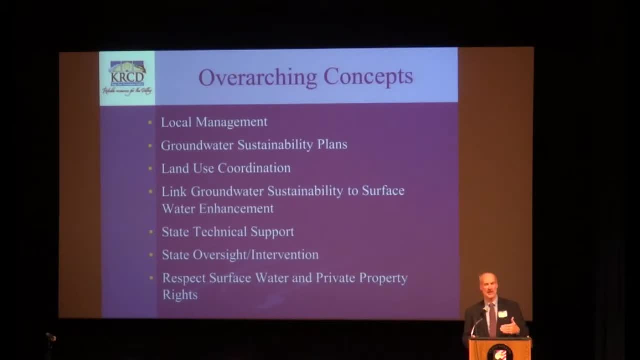 So the concepts included a continuum of management of groundwater at the local level. Remember the state boards out here rattling around thinking that they want to have an increased role in the management of groundwater. Our fear was that we would no longer have the local management authority and responsibility. 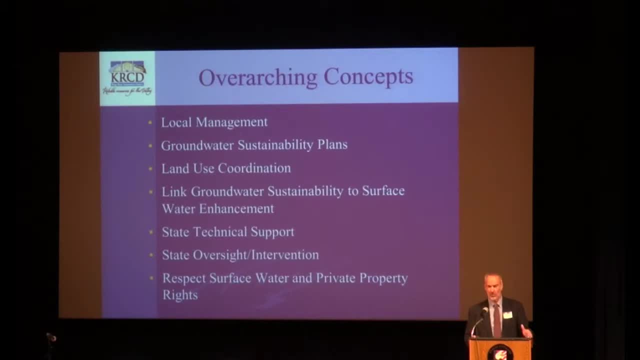 and that a state agency would come in and try to apply a more regulatory approach. There were discussions about raising the bar as to what defines a good groundwater sustainability plan. There were discussions about how do we better connect the land use process with the groundwater management process. 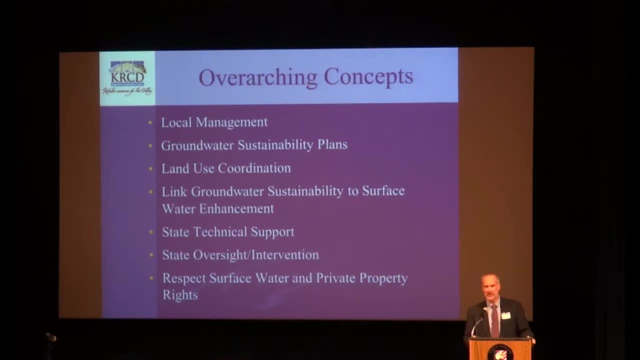 There was already referred to a pretty bold recommendation out of the Association of California Water Agencies that there be an expansion of the Show Me the Water criteria to other users of groundwater, including AG. There was an objective to point out that groundwater sustainability can only be achieved by two pathways. 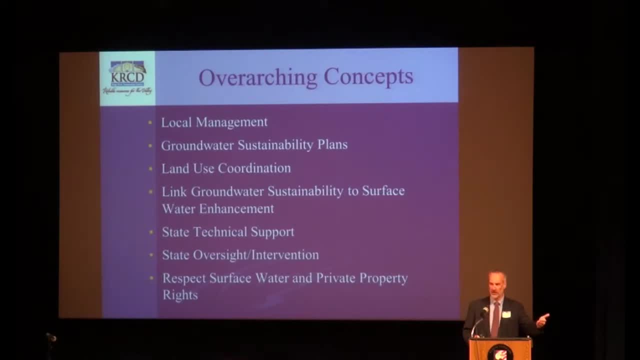 One is reduced demand, which has significant economic harm to a valley that's dependent upon that groundwater, or we can look at enhancing our surface water supplies and achieve sustainability through that pathway. A lot of discussion about the roles of the state agencies and, ultimately, the policy papers defined roles for the Department of Water Resources. 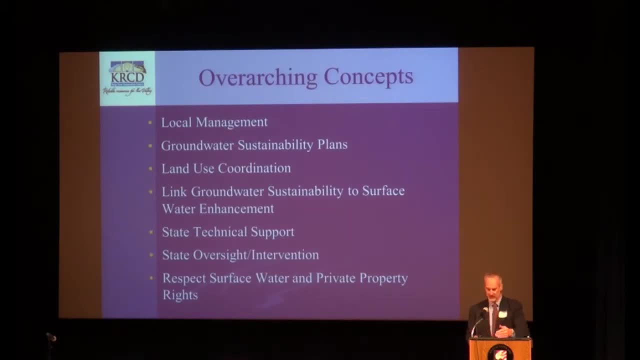 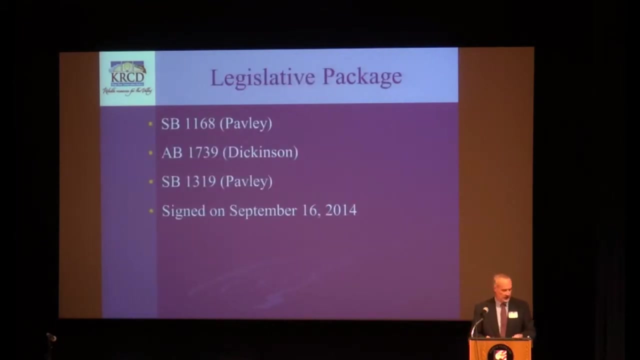 and a separate oversight or intervention role for the state board, with some intent that those intervention points be very clearly defined. and then, finally, a policy objective or a concept was to recognize and respect existing surface water rights and existing private property rights to use groundwater. So the legislative package that came together earlier this year was initially two bills. 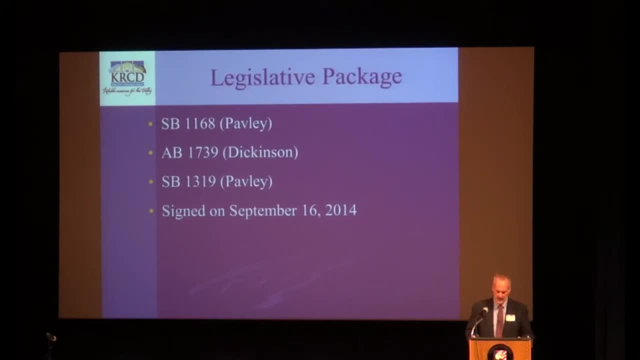 Senator Pavley introduced Senate Bill 1168.. Assemblymember Roger Dickinson introduced AB 1739. The Foundation California Water Foundation and ACWA both worked with these authors, initially individually and then ultimately collectively in what was called a small group process, where the administration came in and we tried to incorporate and negotiate concepts into these two bills. 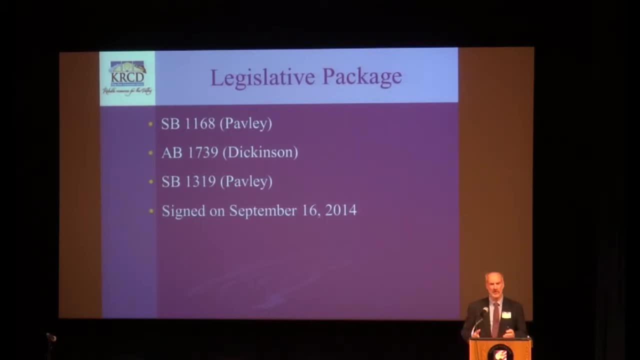 They ultimately were merged And then, since both authors wanted to have some fingerprints on the final product, they split them back out in half and linked the two bills. In the last week of this session- now we're talking late August- it became pretty apparent that some additional changes to the two bills were going to be necessary. 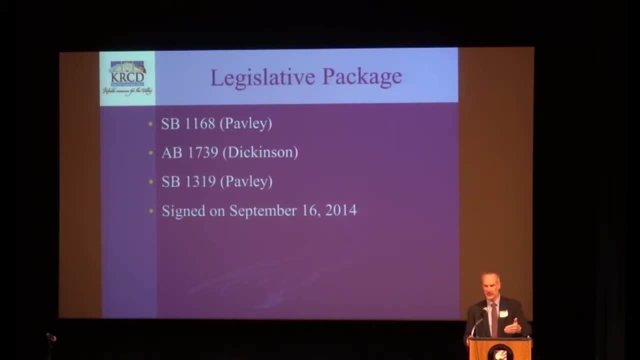 in order to- again we're talking political process here, people- so that in order to get votes to approve the bills, to move the bills out of the legislature, there were some additional concepts that were addressed through Senate Bill 13.. Basically, it missed the deadline for further amendments to the top two bills. 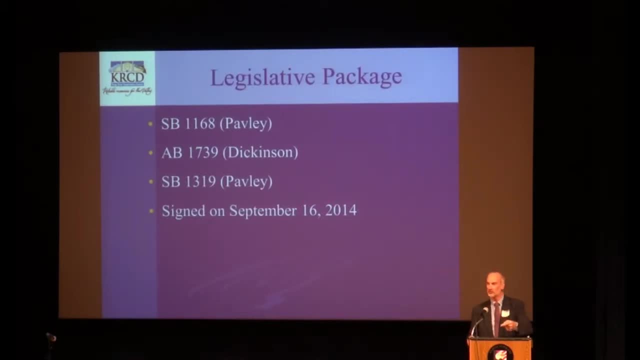 and so the third bill became the vehicle to amend the first two bills and ultimately they were all linked together and became the Sustainable Groundwater Management Act. that was passed out of the legislature next to the last day of session, in late August, and then signed by the governor in September. 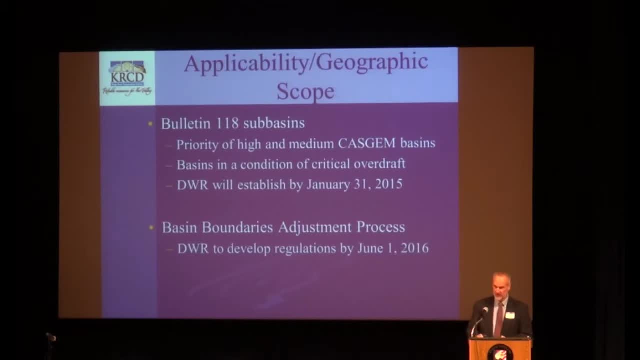 So the scope of the legislation applies literally to every groundwater basin in the state, but there are some prioritizations that occur within the statute. First, any basin that is designated as high or medium priority by criteria that the legislature established in 2009. 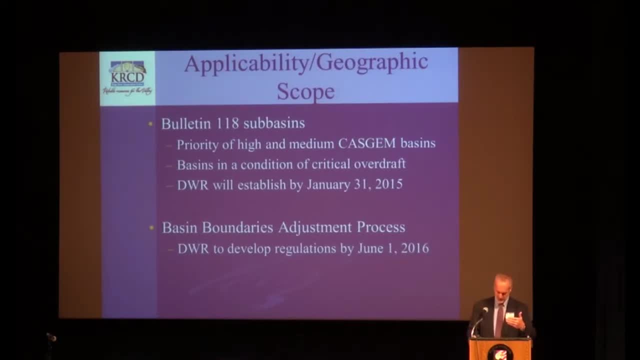 in the Comprehensive Groundwater Elevation Monitoring, or CASGEM, program. those priorities were applied in any basin that's in high or medium priority that is also in a condition of critical overdraft has the first obligation to meet some deadlines, and I'll talk about them. 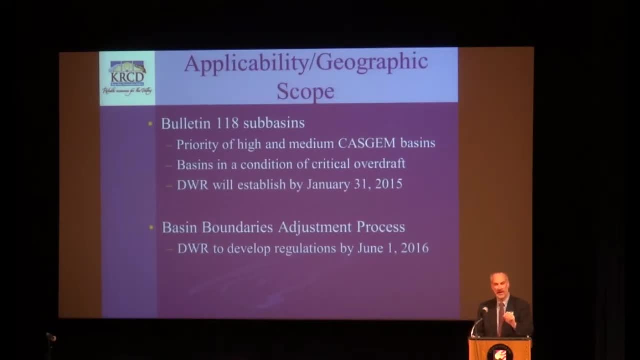 of adopting or creating first a groundwater sustainability agency and then ultimately adopting a groundwater sustainability plan. DWR is supposed to update this CASGEM priority map by the beginning of next year. They've already said publicly that they don't anticipate much change to the map. 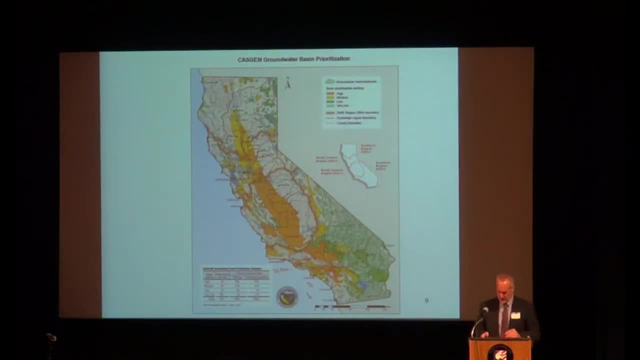 that they released last fall. The most important thing- and I realize this is probably not a great map for you to look at, but the most important thing to recognize- is San Joaquin Valley. dark orange means high priority, So virtually every groundwater sub-basin south of the delta. 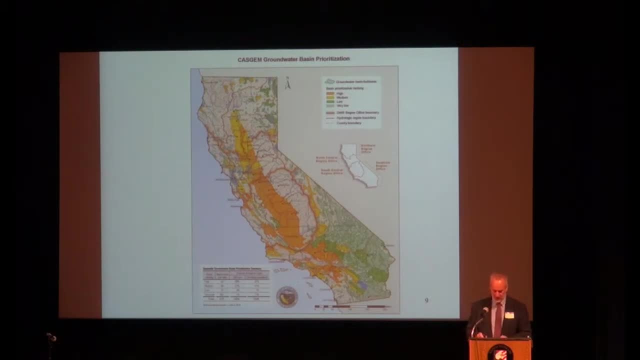 within the San Joaquin Valley are going to have an obligation to comply with this act at the first tier of deadlines. There are processes within the bill that allow agencies to propose boundary adjustments, recognizing that a lot of these groundwater basin boundaries were established decades ago through kind of a geopolitical process. 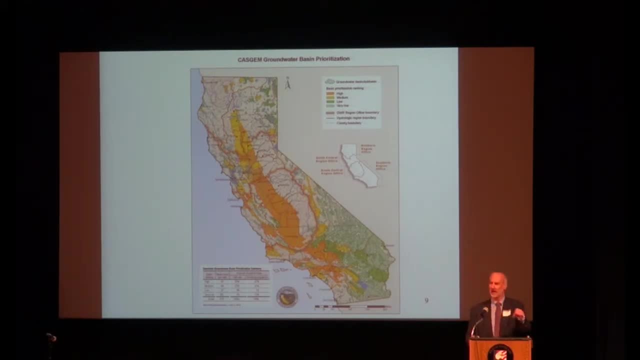 Groundwater magically stops interacting in county lines or water district lines, And so I think one of the things that we'll have to do- and the Department of Water Resources has an obligation to do- is to define criteria upon which local agencies can come in and propose boundary adjustments. 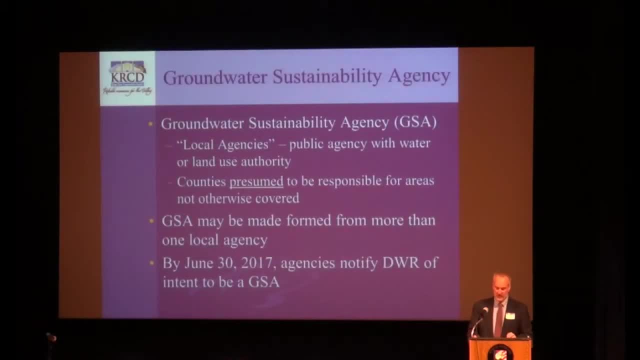 So I mentioned the formation of the GSA. The first step in this process is to create a groundwater sustainability agency, And the legislation does not give priority to any of the existing groundwater management agencies that have been implementing groundwater management plans for the last couple of decades. 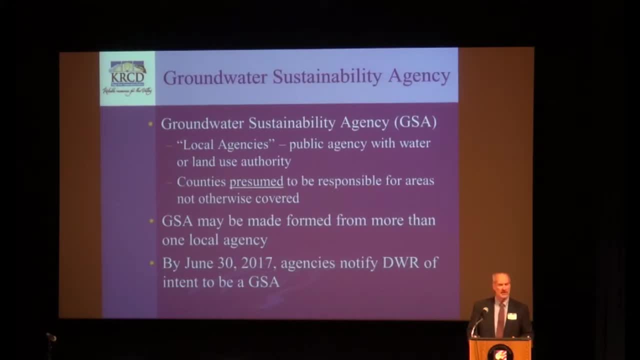 but basically launched what the Department of Water Resources does One of the staff members for Senator Pavley refers to as the food fight option, which means you all get to figure it out at the local level and accomplish the goal by January of 2017,. July of 2017, or there are consequences. Local agencies are authorized to create GSAs, and so a local agency by statute is defined as any public agency with water or land use authority, But the counties have been given an increased responsibility here in the act. 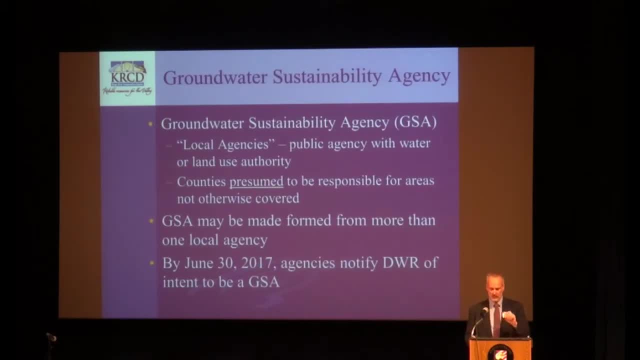 by being designated as the presumed GSA for areas that aren't otherwise managed by some other GSA. It gets pretty confusing to try to figure out who's on first. But there's also a provision within the act that the groundwater sustainability agency can be formed to cover the entire basin. 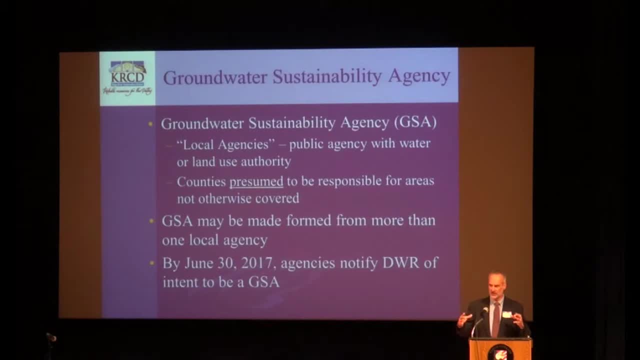 The objective of the act is that each basin be managed to a goal or a standard of sustainability, and yet the act does allow multiple GSAs to be formed within a basin, provided that they demonstrate cooperation and coordination to achieve the basin-level sustainability objective. 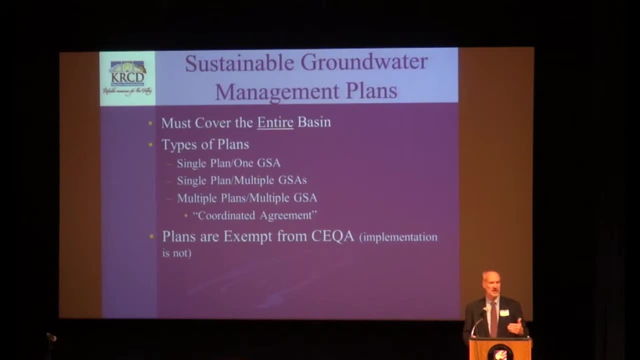 This slide basically speaks to that. There are a number of options that we're already exploring within the Kings Basin that are going to necessitate an ongoing dialogue with the many of you in this room and ultimately decide what is the right type of governance structure that's appropriate. 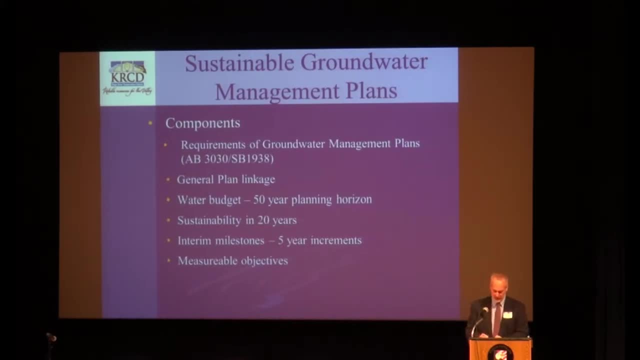 So I'm going to try to speed up here a little bit because I see I'm running short on time. But the requirements of the plans: these are optional requirements under the act that allow groundwater management plans to establish or require a water budget reach a sustainability standard. 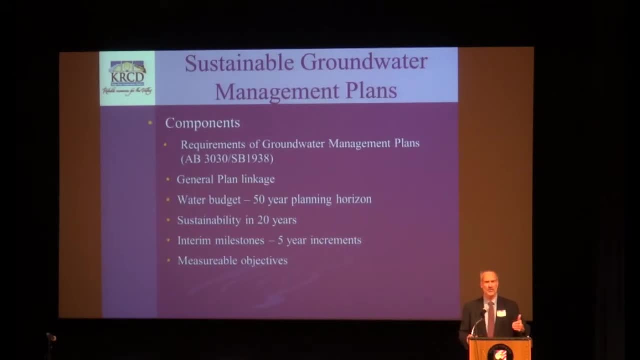 The plans have to have an interim milestone pathway so that DWR can review and assess and determine whether or not you're in compliance. Measurable performance objectives, and all of these build on the existing water code statutes that define what a groundwater management plan looks like. 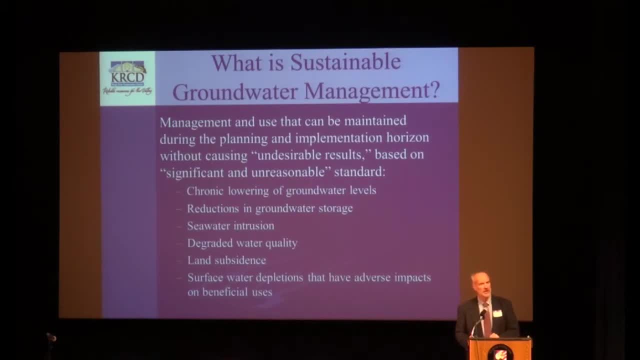 So sustainability- this is a word that we used a lot to claim this or frame this last fall. It's becoming problematic term because it means different things to different people and therefore it's become a target for criticism. But the statute defines sustainable groundwater management. 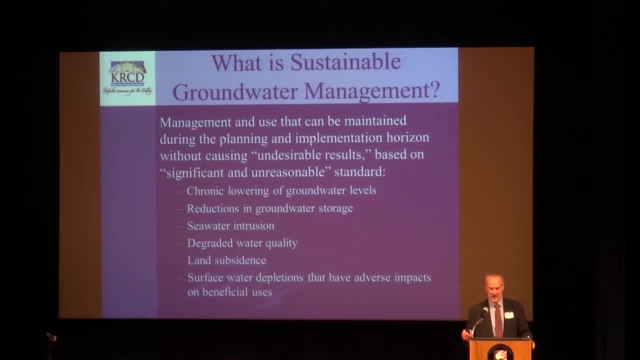 as the management and use of groundwater in a way that can be maintained during a planning and implementation horizon, which is 20 to 50 years, without causing undesirable results. Undesirable results are then further defined in the statute to include the things that you can see here. 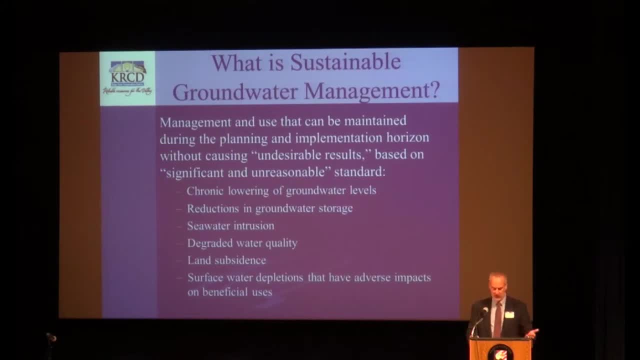 which include chronic lowering of groundwater levels, reduction of storage, degradation of water quality, land subsidence, surface water depletion- that have adverse impact on beneficial uses. It's important to recognize these are not made up concepts. A lot of people believe they are. 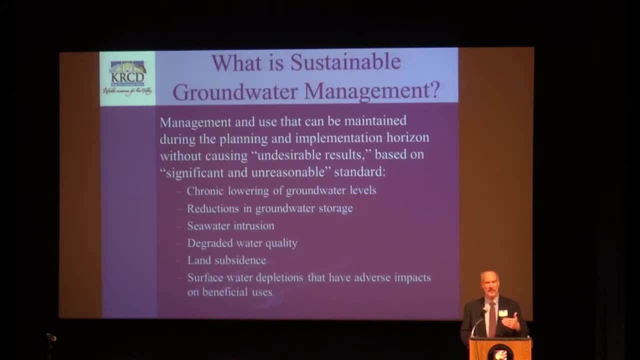 but essentially this section of the act was developed by a number of attorneys that California Water Agencies brought together and were supported by the California Water Foundation in some degree to look at how the courts have typically looked at, when adjudicating a groundwater basin, the criteria to determine. 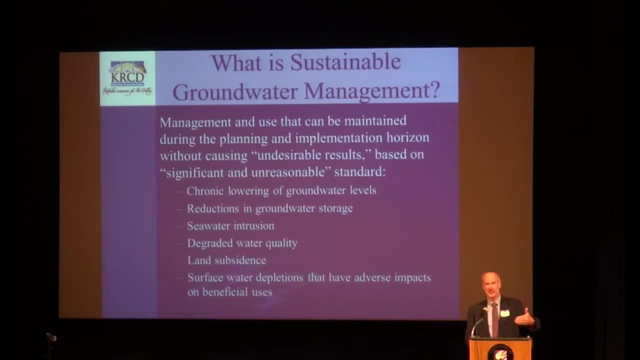 when balance has been achieved And so undesirable results comes out of an appellate court decision. Our group of attorneys tried to define further what undesirable results are by including these criteria and then applying a significant and unreasonable standard against every one of those. It remains to be seen. 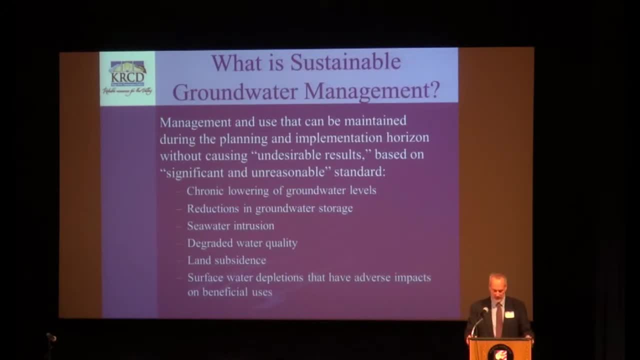 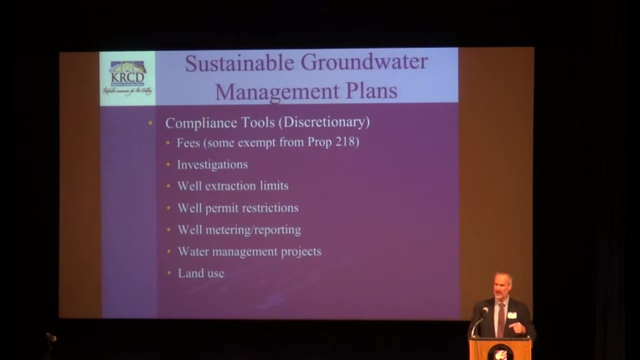 whether we can all agree on what's significant and unreasonable and whether or not results are in fact undesirable. That's part of the dialogue. I think that will occur going forward. So there are some basic tools that have been granted to local groundwater sustainability agencies who adopt groundwater sustainability plans. 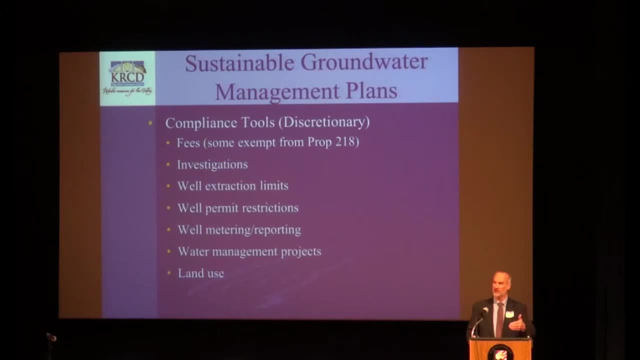 which include the ability to initiate a groundwater management fee, some of which are not subject to Prop 218, which would be required. landowner objection or approval under different structures of those fees allows GSAs to conduct investigations, establish well extraction limits, well permit restrictions. 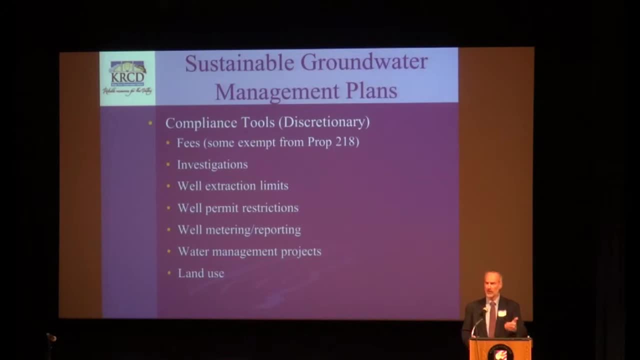 well metering and reporting requirements, pursue groundwater management projects and then coordinate more directly with the land use planning agencies. Important to recognize that how we use these tools at the local level is up to the local agencies. We can ultimately decide that we don't like extraction limits. 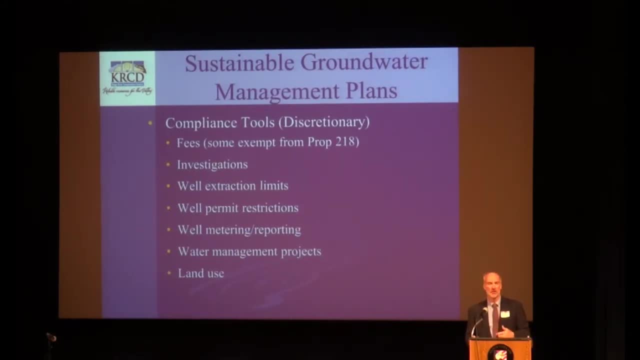 We want to go to a fee structure or we can decide we don't like fee structures. We're going to try to find some other source of revenue to construct water supply enhancement projects. These are discretionary tools that are available for local agencies to apply. So, moving to kind of the state rules, the Department of Water Resources has a couple of specific rules moving forward here In the near future. they have to develop rules and regulations that define how basin boundaries will be adjusted And then by June 1 of 16,. 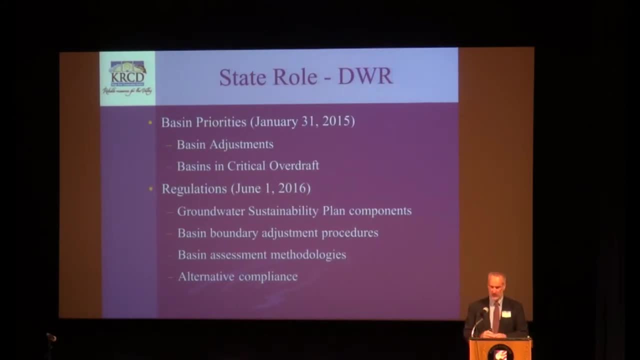 they have to develop rules and regulations that will identify how sustainability plans will be reviewed and deemed compliant with the act for being sustainable. There are best management practice requirements that DWR has to do, And then there are a couple of other things that they've got to define. 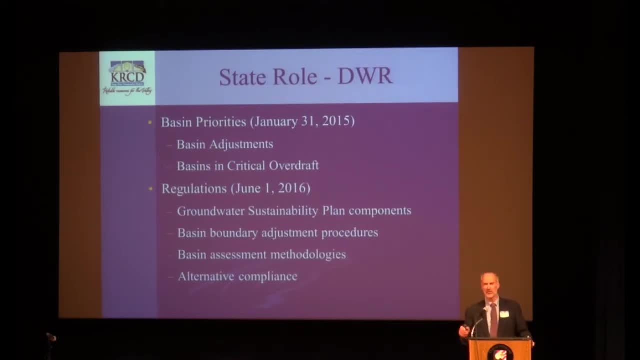 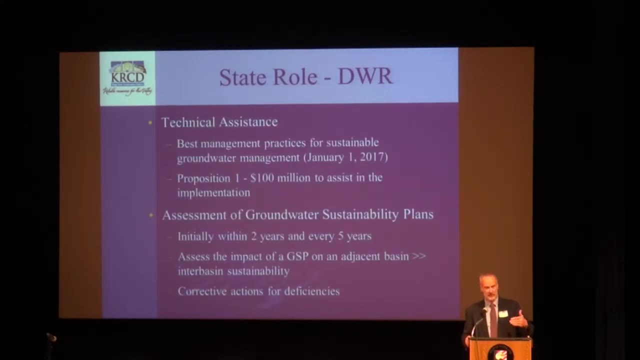 And I suspect they will take a shot at trying to do that And then further clarify what undesirable results means. The department is being funded in part by some existing general fund commitments. Of course Proposition 1 of the water bond frames in this arena. 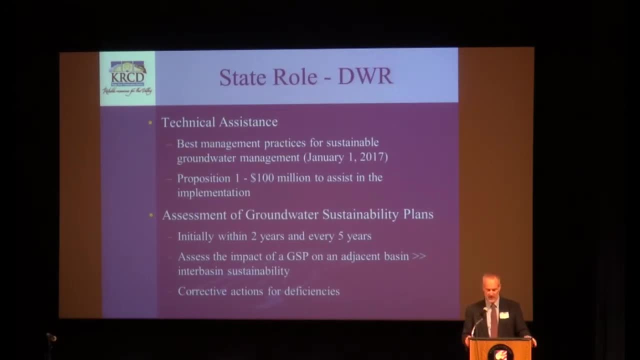 could include some additional funding for implementation that's available through the department to the local GSAs, And then DWR will have to ultimately assess groundwater management plans, identify corrections that need to be made or approve them and then periodically review them If they deem that your plan is not compliant. 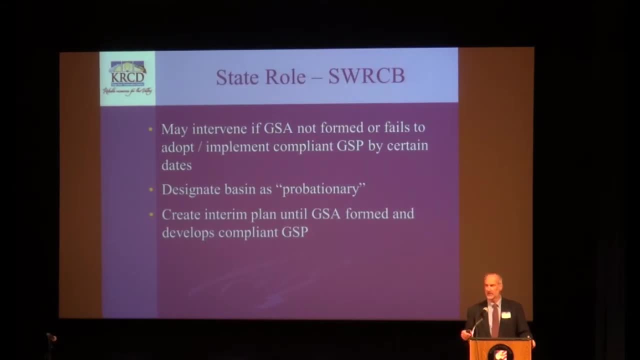 and you fail to correct it. this creates the opportunity, that point where the State Water Resources Control Board can actually intervene, And so here, this slide points out that the board can intervene if the GSA is not formed or fails to adopt a compliant plan. 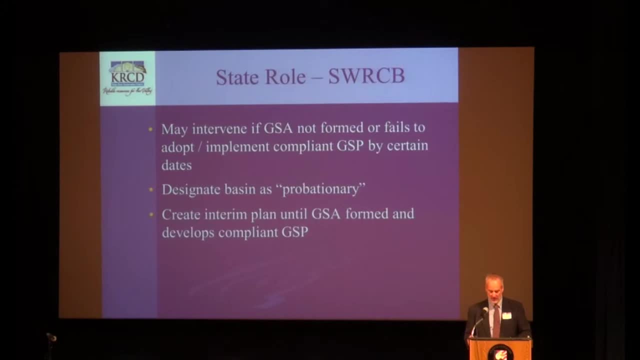 by the defined deadlines in the statute. In that process, the State Board has the ability to designate that area or that basin as probationary and then ultimately create an interim plan until the locals decide that they want to implement their plan. Important to recognize that the State Board's criteria 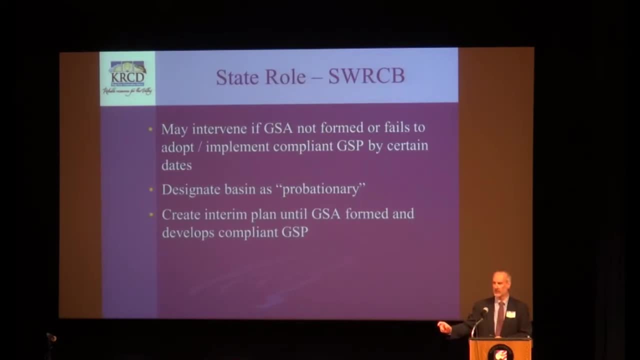 for an interim plan are not the criteria for a groundwater sustainability plan. The State Board can simply come in and say: we believe that your safe yield is X, and so you only get to pump X until you figure out how to manage your plan under a sustainability objective. 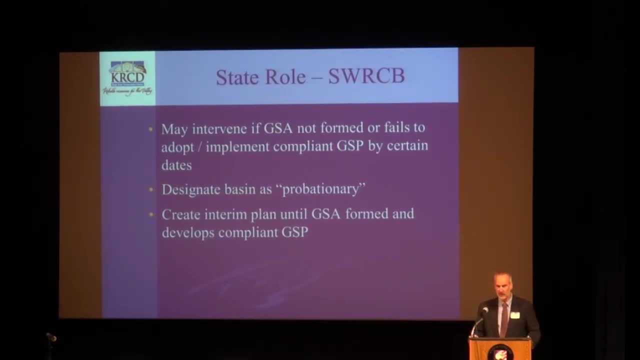 at the local level. So not a good alternative, frankly, to find ourselves in a place where we've been unable to reach agreement and invite the State Board to come in. There are some timelines for State Board intervention. Remember I said at the beginning: 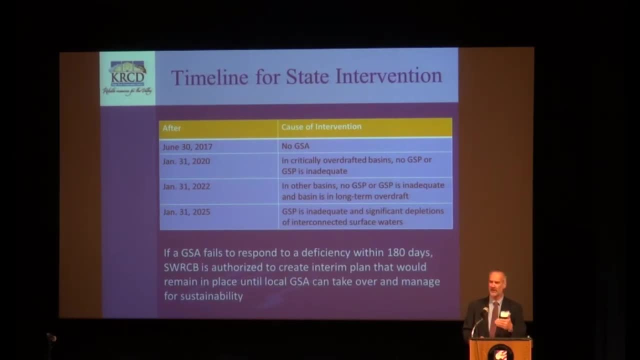 that we wanted some finite, defined criteria That would determine when the Board could come in. My objective was to push them back to the back end of this process and to some degree I think that was achieved. So they can't act until a GSA has failed. to be formed by June 30th of 17,. or if, depending on what status your groundwater basin is in- medium or high priority, critical overdraft or not- you have to adopt your groundwater sustainability plan by June 30th or by January of 20,. 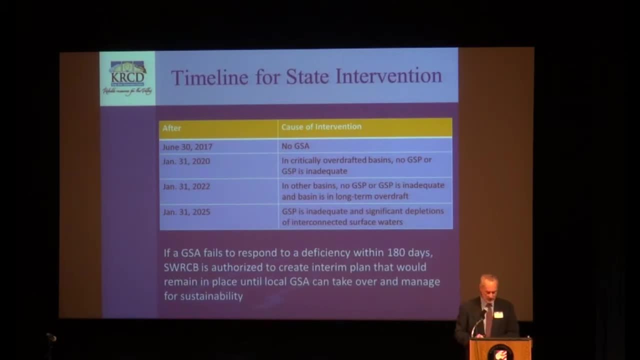 or January of 22, or even January of 25.. There's again you can see here at the bottom is that there's an identified deficiency in this intervention process that locals still have the ability to cure before the State Board steps in and initiates an interim plan. 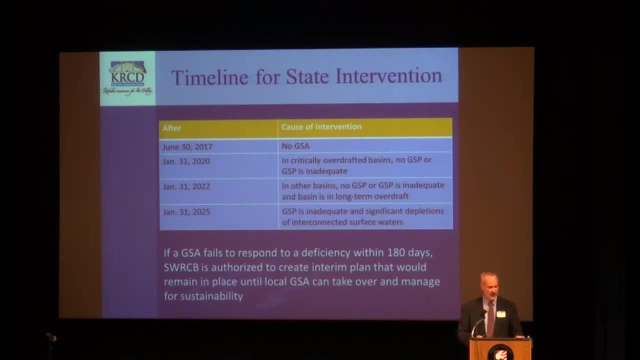 I refer to all of this. as you know, we have our hands on the wheel at the local agency level. We can decide how long we want to steer, whether or not we want to get ourselves to a place that keeps the State Board out of our business. 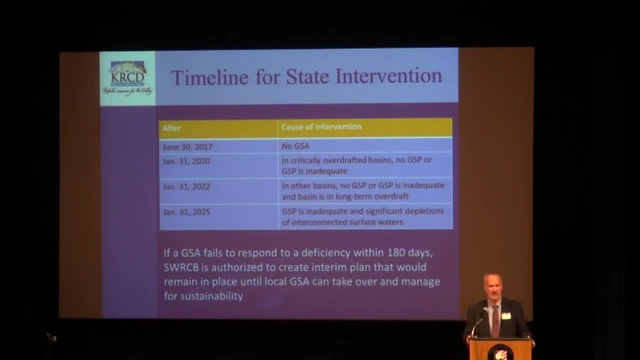 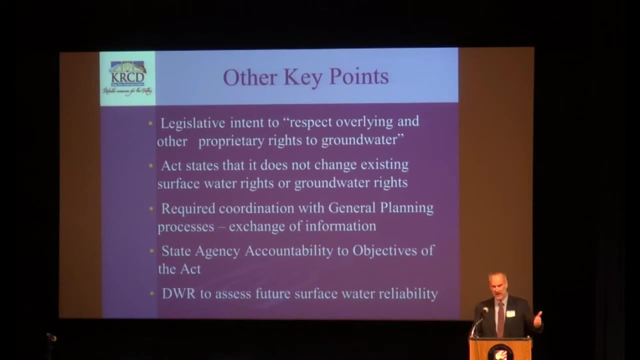 Remains to be seen if that's possible. So just a couple of other key points to identify, looking back about those objectives. The legislation includes a statement of intent to respect overlying and other proprietary rights to groundwater. states that it is not intended. 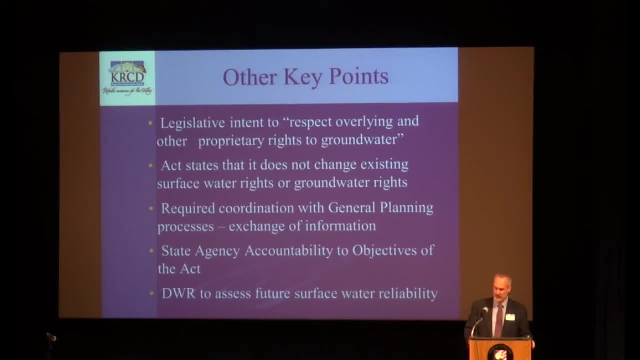 to affect surface water rights or groundwater rights to the extent they've been defined, and it's not intended to affect the quality of the water that's being used. So again, it's not intended to affect the quality of the water that's being used. 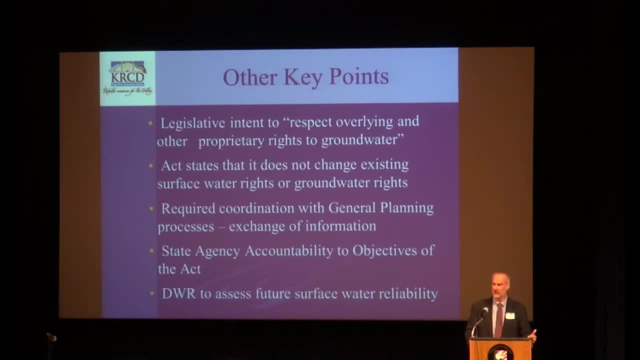 It's not intended to affect the quality of the water that's being used. It's not intended to affect the quality of the water that's being used. The census application supports the 가 in this approval. that requires some coordination with the land use agencies. 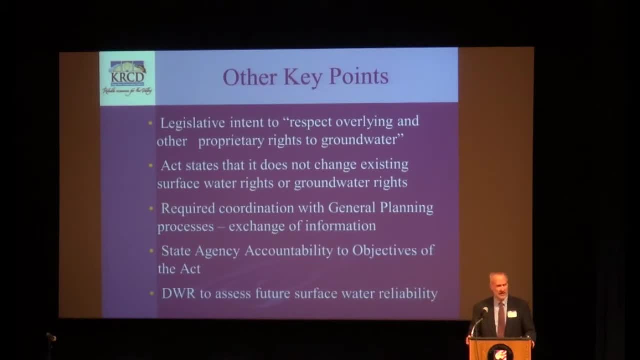 but it's really through an exchange of information. There's not authority for a groundwater management plan in order to write a general Jinra woman or anything that would restrict power of lndo, The counties and the place of decision land use planning process that says as the state makes a decision moving forward, they have to consider the 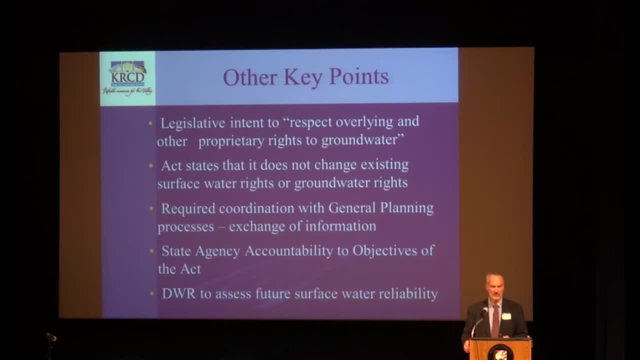 objectives of sustainable groundwater management as they make those decisions. This can be important in water quality regulation and establishing flow standards and making a lot of decisions, including, perhaps, enforcement of the volumetric pricing and volumetric measurement requirements that come out under SB 7x7 from 2009 that a lot of our local agencies are continuing to try to. 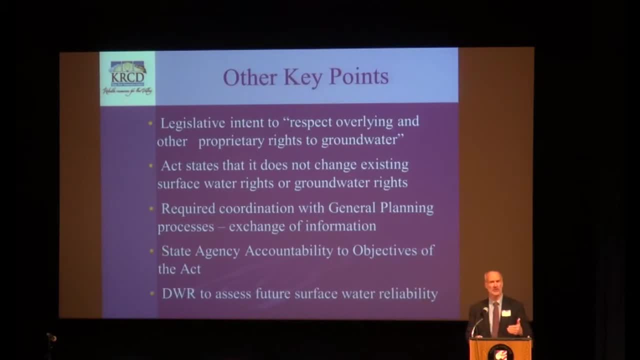 deal with. And then DWR ultimately has to issue a report of future surface water supply reliability, which would be an interesting process. to have them look at the California Water Action Plan and all of those things that were on that schedule and then determine how do they translate to more supply and they 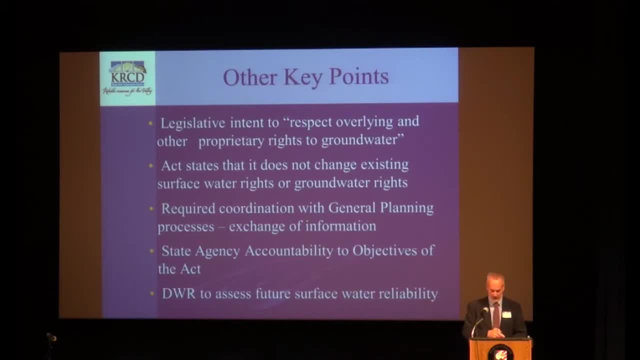 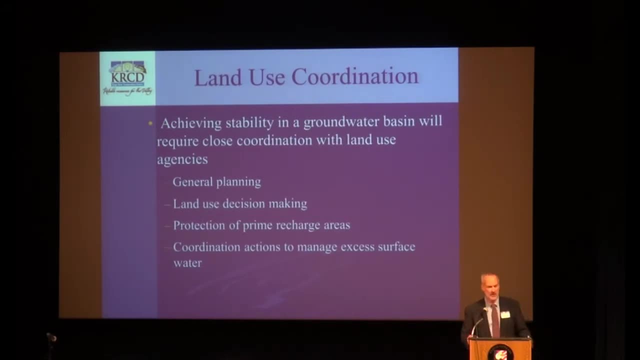 translate to sustainable management of the groundwater basin. There's obviously going to be a significant requirement to better engage the land use planning agencies. We've talked about that in the general planning, the land use decision-making, the protection of prime recharge areas and the coordination of actions to capture excess surface flows when 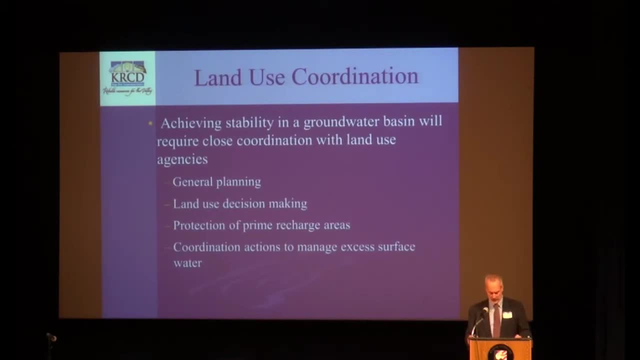 they're available. So, again, you know that new dialogue that I referred to in the opening comments. Finally, just to kind of talk about next steps, I think that the first thing that we're doing, and we continue to do pretty aggressively, is initiate a local outreach and communication strategy to 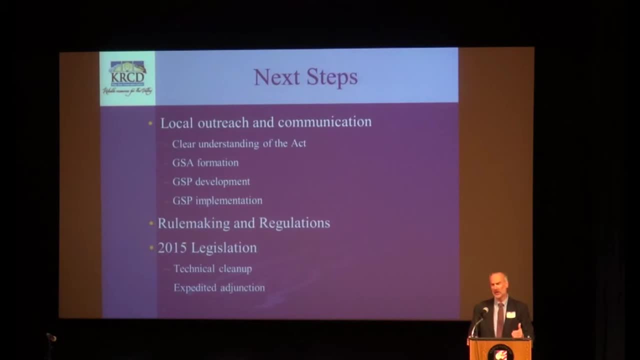 help people clearly understand what the Act is and what the Act isn't. There's a lot of misinformation, a lot of rhetoric out there as to what the Act actually does. I think we need to really get ourselves to a common understanding of what it. 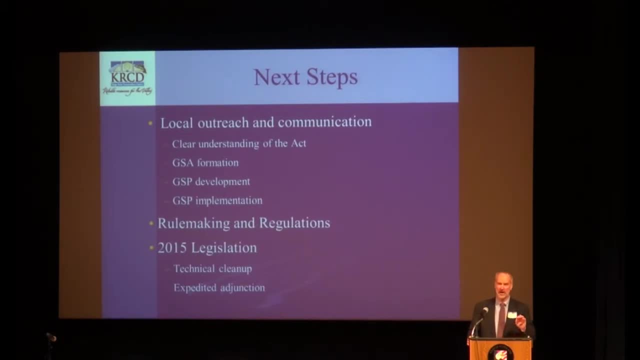 what it, what it clearly requires of us, and then work together to collaboratively to decide whether or not we want to try to forming a groundwater sustainability agency or agencies to cover the planning area, adopt, develop and implement a groundwater sustainability plan and get ourselves on. 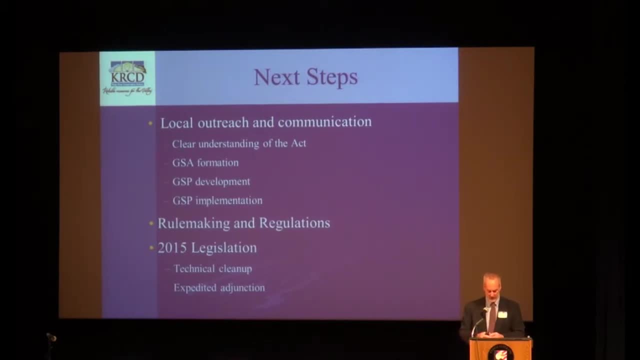 that pathway to sustainability that keeps the state out of an interim action. What DWR is going to do with rulemaking and regulations is going to be critical, because it will define a lot of the terms and conditions that a lot of people are struggling with in the Act and then, ultimately, I 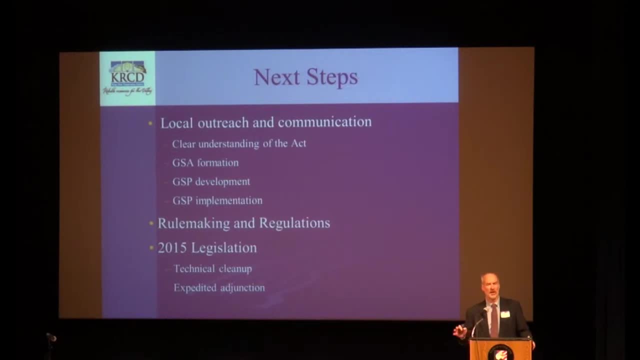 think there's already some discussion about two types of cleanup or two types of legislation Next year. I've heard them referred to as number one, cleanup or technical correction, and number two, unfinished business. It's the unfinished business that I'm worried about. What are they going to do now? 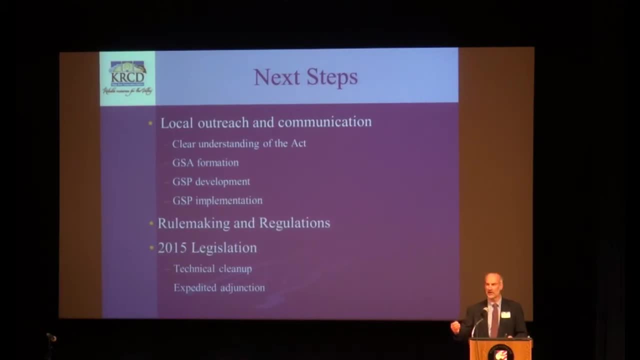 There were a lot of things that were resolved and left on the table. I think there's some discussion about trying to clean up the adjudicatory processes that the courts used to determine acreage property rights under the formula that Ellen referred to. There's a real little clear direction today as to what a judge 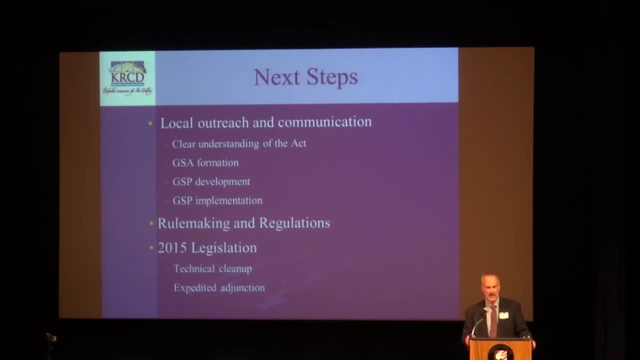 should do when he initiates an adjudicatory process and whether or not he's going to do the correlative equal per acre approach. or look more at the way we do first in time first amount of money and whether or not he is going to do the correlative equal per acre approach. or look more at the kind of the way we do first in time first amount of money. 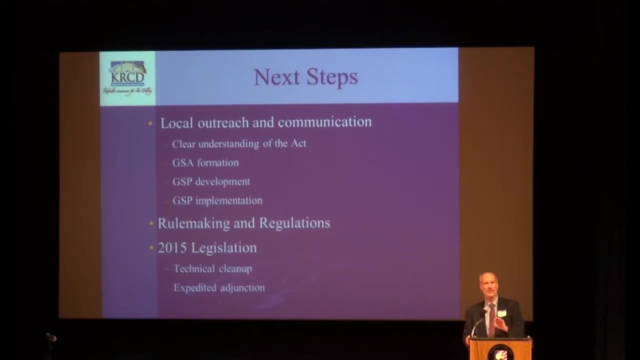 for surface water. so there's a lot of discussion about whether or not we can put the legislation together that provides a clearer path to adjudication. let me close by saying there's there's kind of three options here, and status quo is not one of them. recognize that the bill's been. 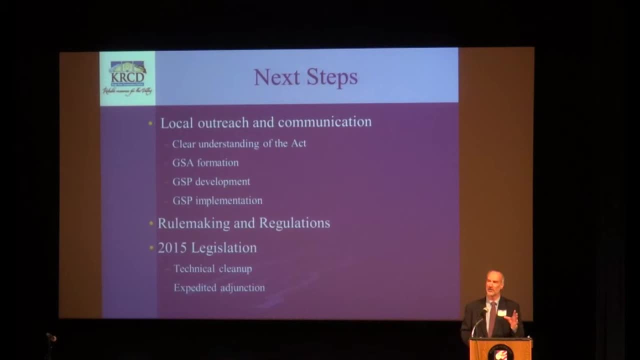 passed, and even without the passage of the bill, i think we were on pathway in this state to either expanded state intervention and control of groundwater resources and in many cases in an ad, in a way that's adverse to our local interests. so that's one path is state involvement, participation. 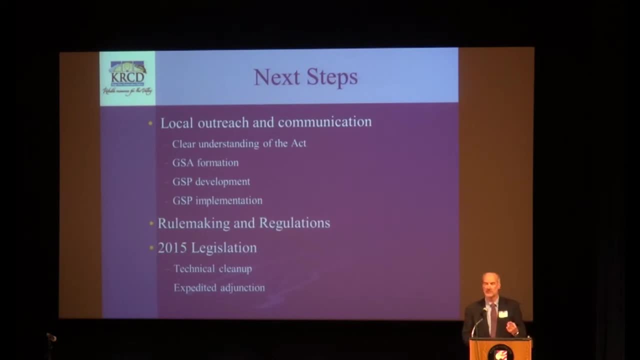 path number two is litigation, and litigation ultimately will lead to, in my opinion, adjudication. we can challenge a lot of different things, but ultimately it's this, is this issue gets perfected in front of a judge. i think it ultimately becomes a question of how much resource do i have to spread across how many beneficiary uses? 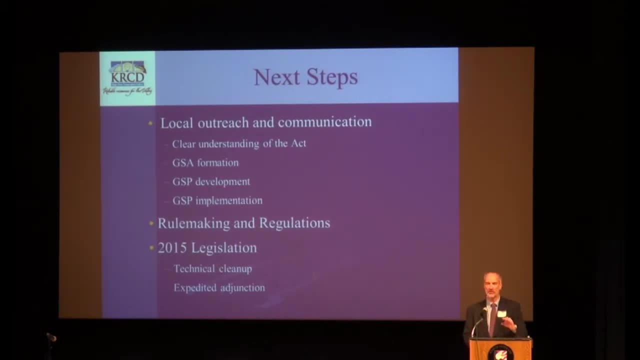 and what do i do to allocate that restricted resource in that area? the third option we have is the pathway that the act spells out, and that is to come together at the local level and create groundwater sustainability plans that are focused on building resource. i'm focused on protecting the 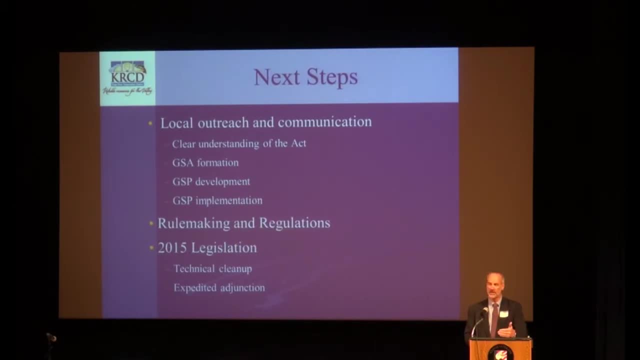 the economic and beneficial uses that are important to each sub-region and find that in a local, balanced way to avoid path one and path two. so with that, um, appreciate your attention again. i probably have time for a question or two, um martin. the question that i have, dave, is in regards 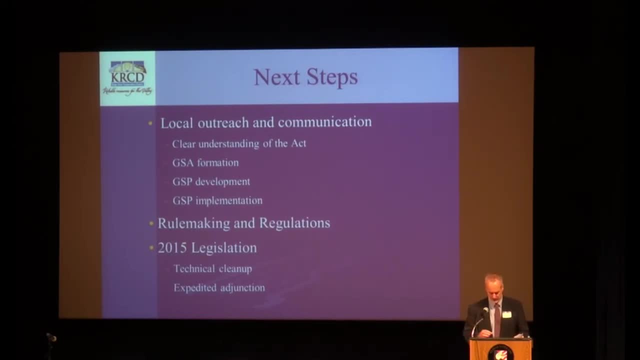 to, um, whether they're going to use tort loop. uh, for the historical, i think that there are many entities in the state that are using groundwater right now. that would say, well, we want historical from an urban perspective. what that would, what that would, what i would then. 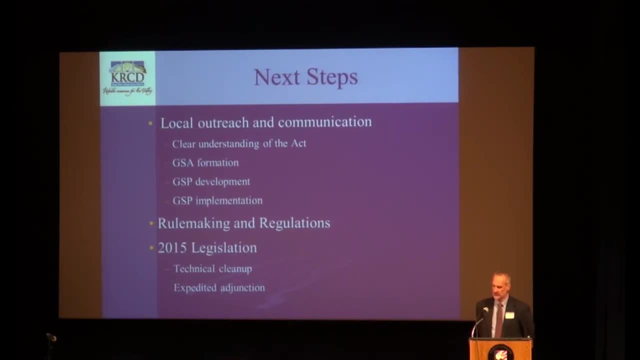 recommend- if i was recommending urban- is: get rid of your drought plan, get rid of all of your conservation measures that you've implemented, because you're going to be restricted in whatever amount you're pumping right now. you won't be allowed to expand your sphere of influence or 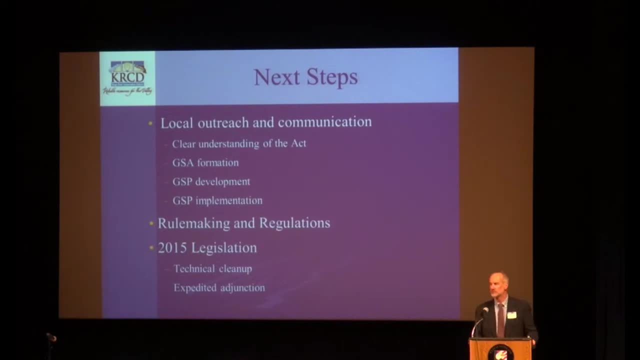 an additional business. so pump as much groundwater as you can right now because you need to establish your historic right. so i think there needs to be some conversation early on about how that's going to be handled. so if you don't have an unintended consequence that is, you know, negative to the correction we're trying to get, yeah, i would agree. 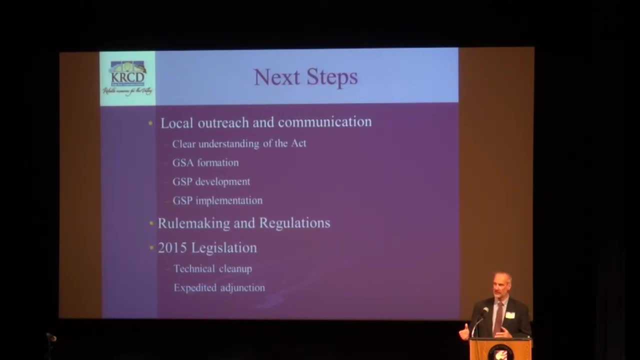 i mean, i think what you do is is emphasize the uncertain future that an adjudicatory process lays out for us. somebody who thinks that's the pathway. um, and you know, again, i'm a policy guy. there may be some attorneys in the room that are experts on adjudicatory processes that we could talk with. 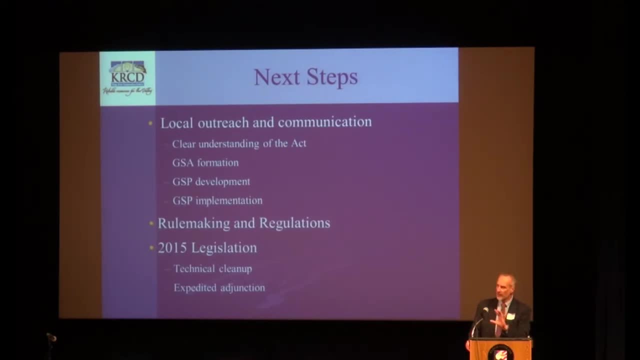 i will point out. well again, i think from my perspective, the courts have been pretty inconsistent in this area and, as i've talked to various stakeholders throughout the state in the last several months, there are some who firmly believe that it's it's a flat per acre. 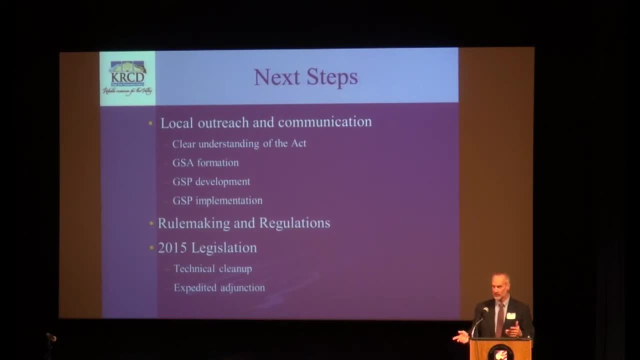 location or limited resource. and then there are others who believe- and, of course, have been on both sides of this issue- it's a personal time first and right, showing how much you've used historically. you'll get a percentage of that moving forward. um, so it's critical that we have 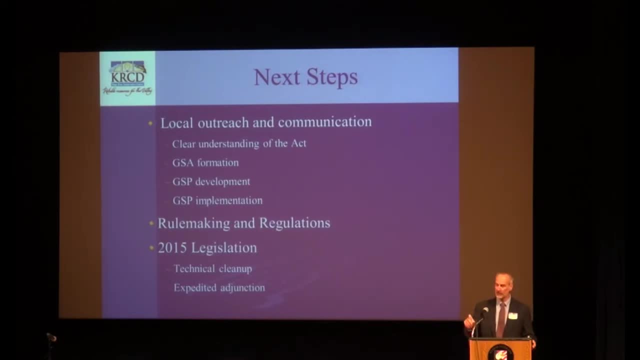 a better understanding of how that works and then a policy discussion about whether or not we can frame it differently through legislation. there is a senate hearing scheduled for january 20th in sacramento that's going to initiate some discussion about how property rights to groundwater are defined, determined and what are the issues that go into these processes. 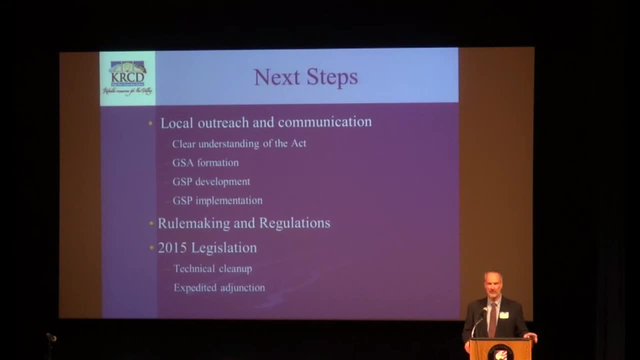 and i think that would be pretty informative to try to eliminate some of these things. any other questions? yes, david, it says that there's no restriction or change on groundwater rights. yet you're talking about either allocation of water or feed structure. that, seems to me, is a change in. 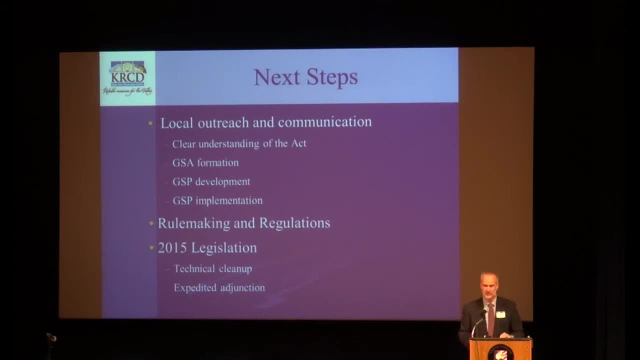 groundwater rights and that's what my constituents are telling me. i've heard the argument: um, i will. i will tell you from my perspective. i think there is a significant misunderstanding of what rights to groundwater are. some people will tell you that your right to groundwater is to pump whatever you can use on your overlying property. 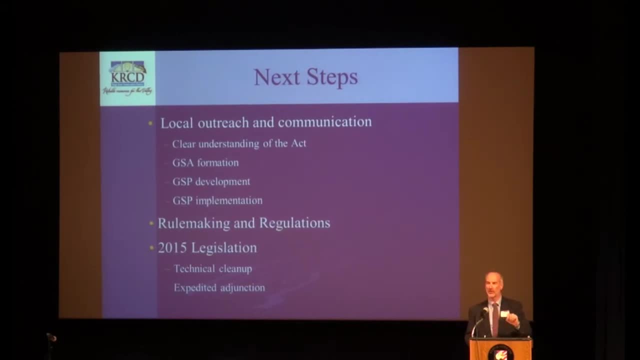 i would add a qualifier to that: so long as it's within the safe yield of the basin and doesn't harm your neighbor, because that's how the courts have determined safe or sustainable yield. so there needs to be, first of all, a significant discussion about what is actually a groundwater right. 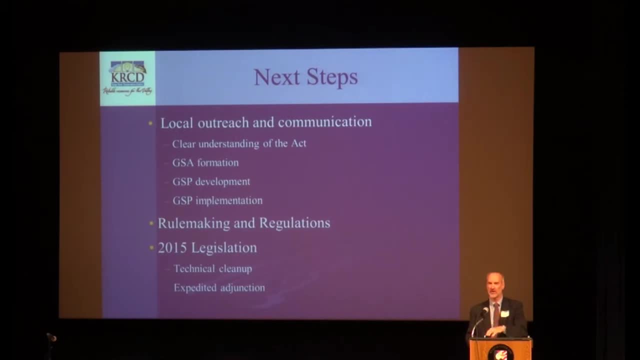 right and then a discussion of how do we allocate that, that that right, amongst the users within a basin. i would i would tell you that a court's going to look at it one way or another. i think a groundwater sustainability agency has the ability to explore and make decisions that are. 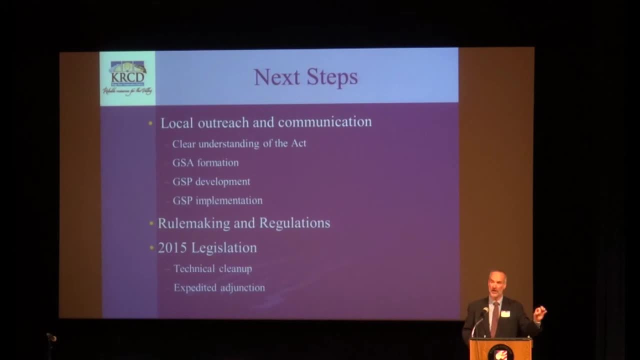 that are protective of their local interests that the court might not perhaps fulfill. it has the authority or need to do. but clearly, you know, an attempt to restrict a pumping right or charge a cost related to the use of that groundwater some people are going to feel is infringing upon their property right. i think we need to have a better understanding. 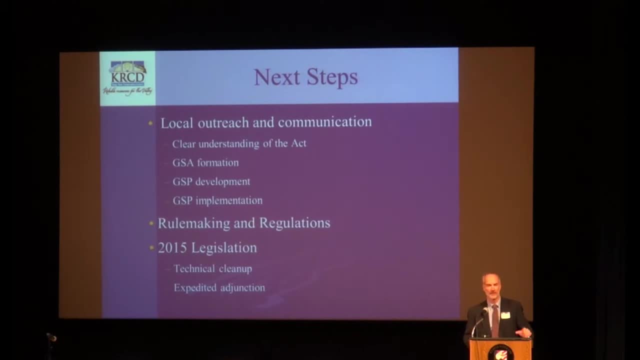 of what that right actually is to be honest. one more question, or we can move on. okay, thank you um.